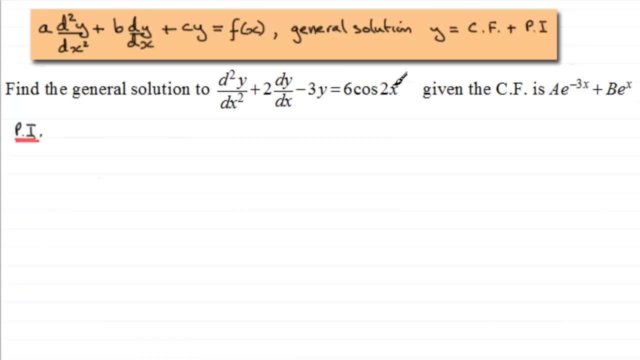 it's 6 cos 2x or even 6 sin 2x, then the particular integral that we use is to let y equal any constant, let's say lambda. then we have cos 2x. But it doesn't stop there. 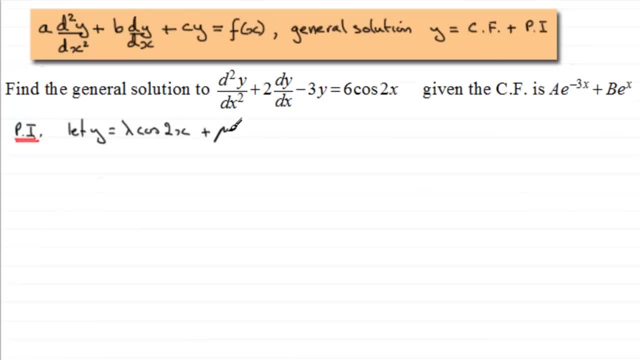 We put plus another constant, let's say mu, and then we multiply that with sin 2x, So I could have had, say, 6 sin 3x here rather than cos 2x, 6 sin 3x, My particular integral. 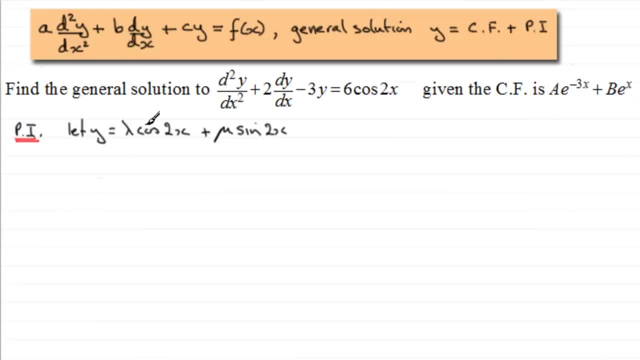 would have been of the form y equals lambda cos 3x plus mu sin 3x. So, as I say, it doesn't matter whether you've got cosine here or sine. Go for this style, Okay. well, on that basis, we do as we've done many times before in. 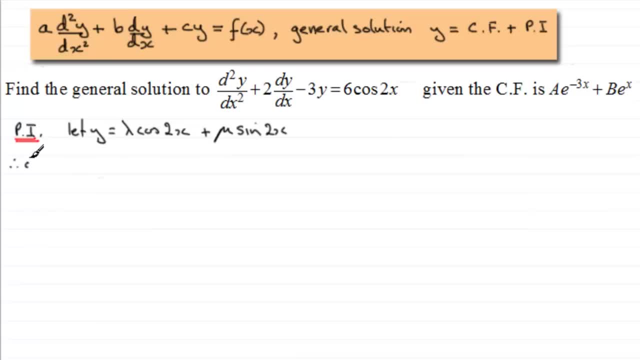 these types of questions, if you've been looking at them, and that is to find dy by dx and then the second differential, and we'll substitute those values into the equation. Okay, so for this one, if we differentiate y with respect to x for this first term, here we're going. 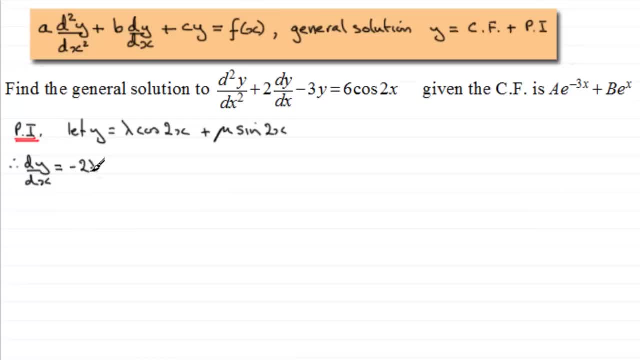 to get minus, Minus 2 lambda sin 2x. And then, when we differentiate the second term here with respect to x, we're going to get plus 2 mu cos 2x. Okay, so that's dy by dx. Now we need the second differential. 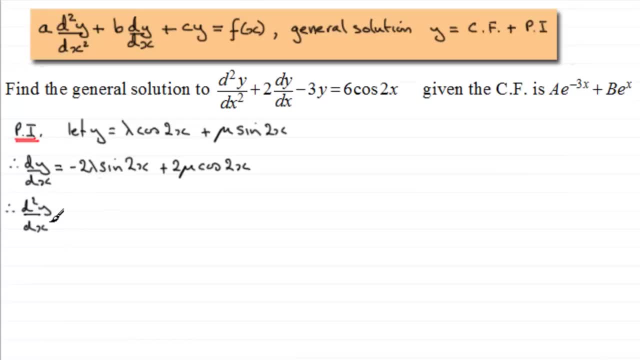 d2y by dx squared. So differentiating the first term here is going to give us minus 4 lambda cos 2x. And then, if we differentiate this term here, we're going to get minus 4 mu sin 2x. Okay, so we've got y dy dx and d2y by dx squared Now because 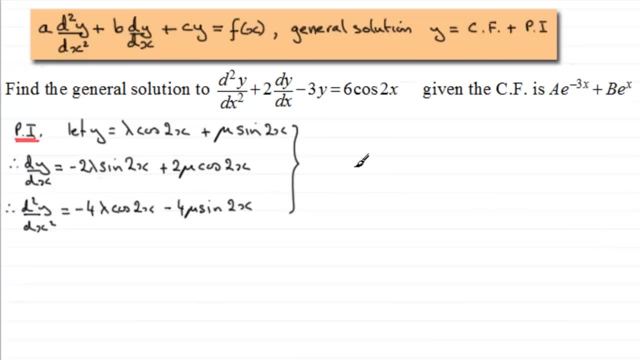 there's lack of room here. what I'm going to do is we'll substitute these values in to this equation up here. We'll call it 1.. Okay, so we'll sub into 1.. Okay, sub into 1.. But what we're going to have now is that, for this term minus 3y, let's just treble all. 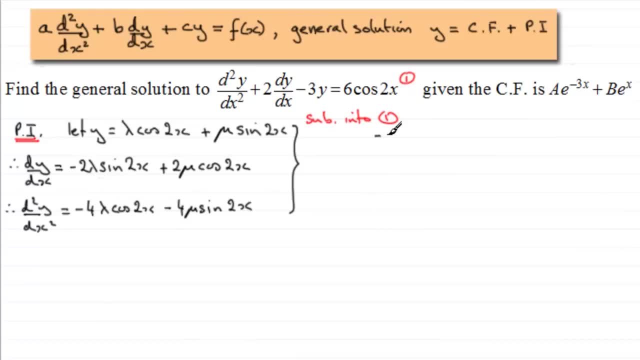 these values here. So we've got that minus 3y equals. well, times this by minus 3.. We're going to get minus 3.. lambda cos 2x. and if we times this term by minus 3, we get minus 3, mu sine 2x. 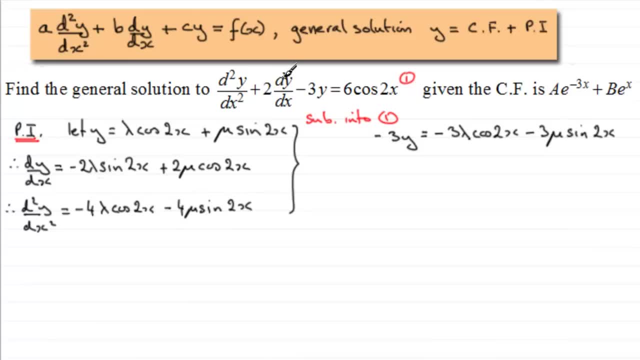 Next, we've got to add two lots of dy by dx. so if we do two lots of dy by dx, 2dy by dx, what are we going to get for this one? Well, if we double each of these terms, what I'm going to do is take this term first so that I can work in columns here, and we'll have 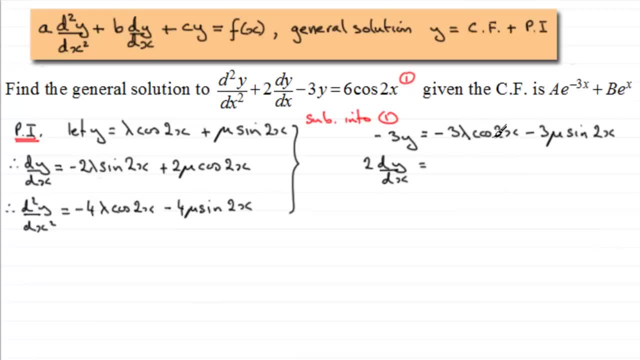 this first column as the cos 2x terms. So I'll double this term. so we've got 4 mu cos 2x, 4 mu cos 2x, and if I double this term we're going to have 4 mu cos 2x. 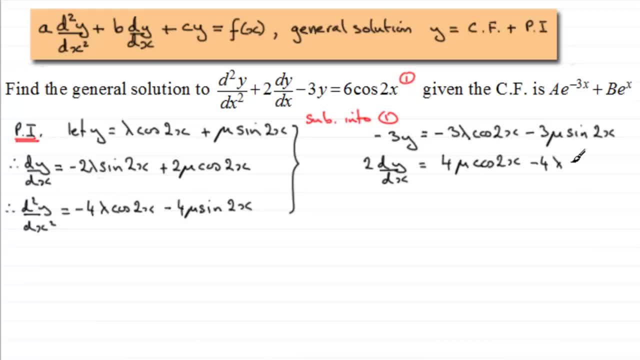 Minus 4 lambda sine 2x and finally we've got dy by dx squared. We don't have to do anything to that, so let's just copy that in: dy by dx squared. We'll take it in the order that it's there. so we've got minus 4 lambda cos 2x and then minus 4 mu sine 2x. 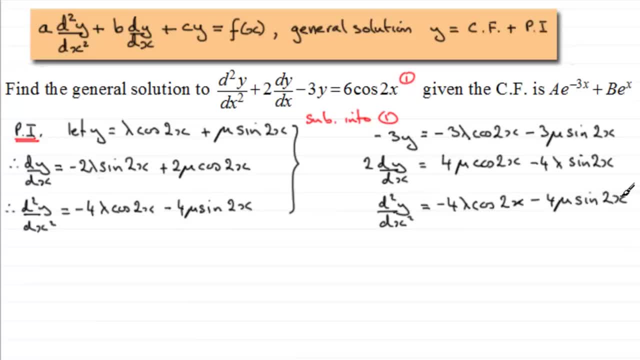 Okay, well, if we now add these terms together- okay, we add these terms together- then we can see that if we compare the cos 2x terms, looking at this first column here, we've got a total of minus 7 lambda, plus 4 mu, and that must equal the 6.. So let's just border this off. 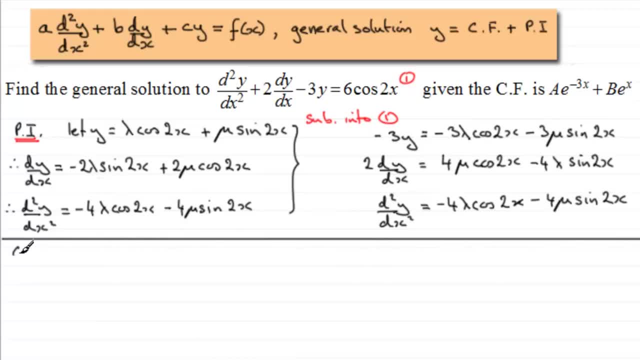 okay and we'll say: well, compare the cos 2x terms. We'll look at the coefficients there. So, as I say, we've got minus 3 lambda, minus 4 lambda, that's minus 7 lambda, and then plus the 4 mu and that must equal the 6 here. 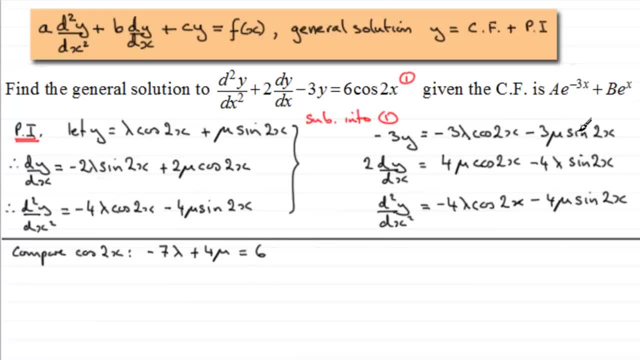 Let's also compare now the coins coefficients of sine 2x. so just write that here. compare sine 2x coefficients and again, if we do this, what we've got is minus 4 lambda, and for the mu we've got minus 3 mu minus. 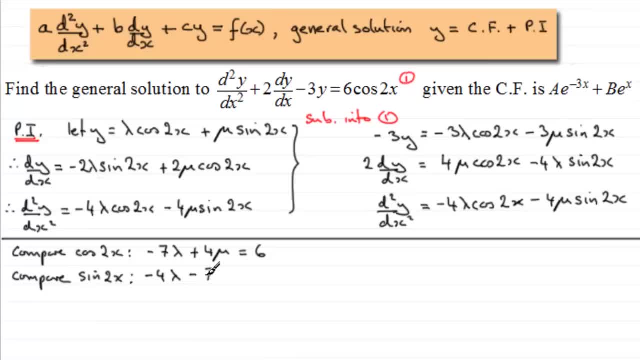 4 mu, that's minus 7 mu. and we've got no terms on the right hand side that are sine 2x, so the coefficients of those would be 0. then now, if you were to solve these two simultaneous equations for lambda and mu, you'd find that lambda turns out to be minus 42 over 65. I'll. 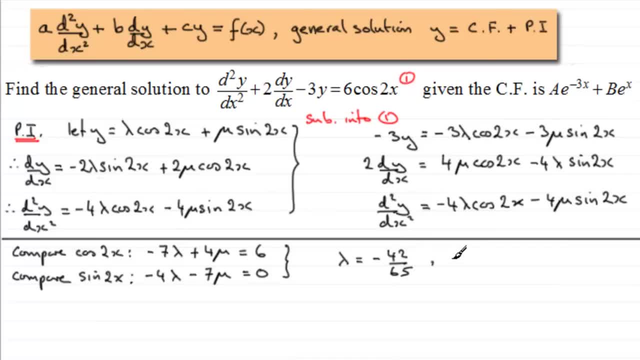 leave it up to you to just work that out. you and mu will turn out to be 24 over 65. so what that means now is that the particular integral pi for short then- is going to be what we've got it as being lambda cos 2x. so it's going to be. 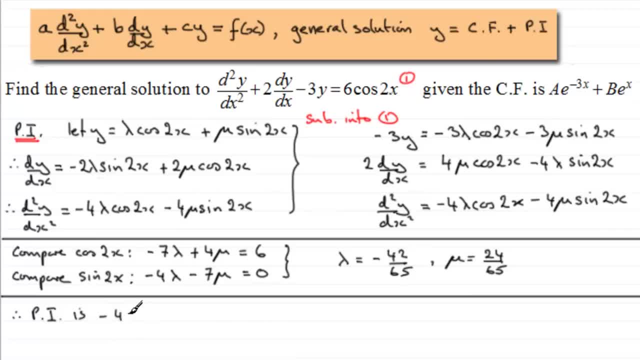 minus 42, 65th cos 2x, and then we've got plus mu sine 2x, so it's plus 24, 65th of sine 2x, and that gives us our particular integral. so what we have next is the general solution. I'll just abbreviate that to gs and 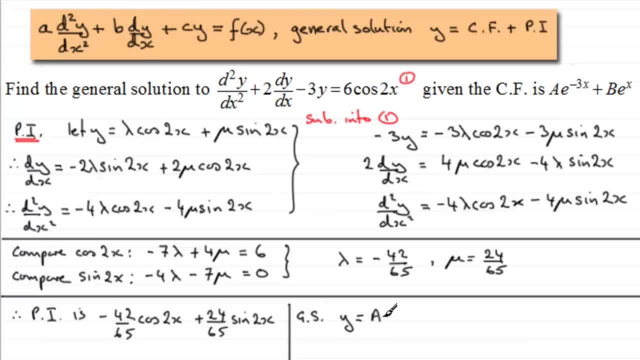 that's going to be the complementary function, which is a: e to the power minus 3x, plus b? e to the power x, and then to that we just have to add our particular integral. so instead of it being a plus, we've now really got minus 42, 65th then of cos 2x, and then plus 24, 65th of sine 2x. okay, so I hope that's.